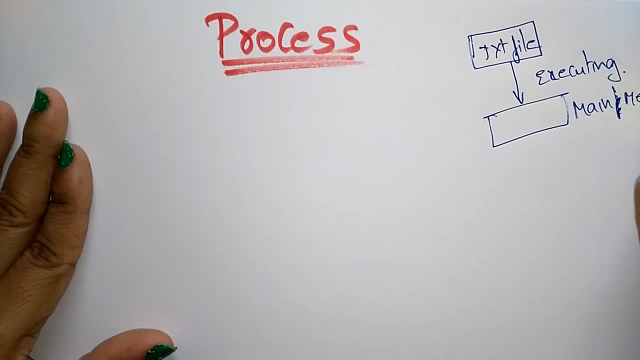 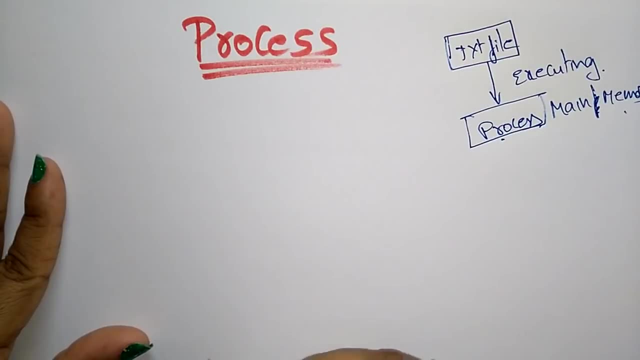 if the program enters into main memory, then you call it as a process. So starting it is a program. When it enter into the main memory, then we call it as a process. Means that program is divided into different modules and each module you call it as a process. Okay, so let me explain. 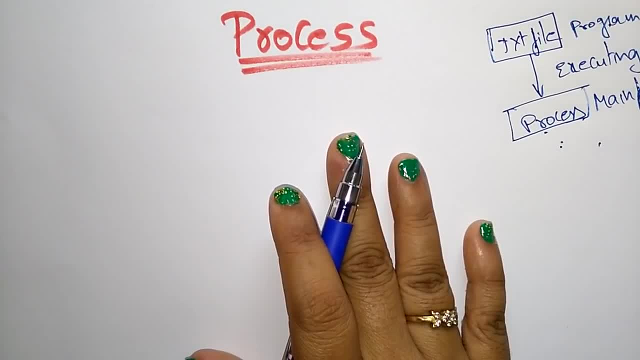 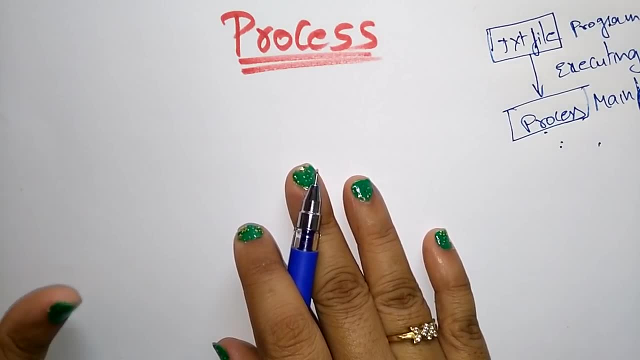 clearly, A process is just, it is a fundamental to the structure of operating system. So, whatever operating system you have taken, so every operating system, the process is a fundamental to the structure of operating system. So every operating system, the process is a fundamental to the. 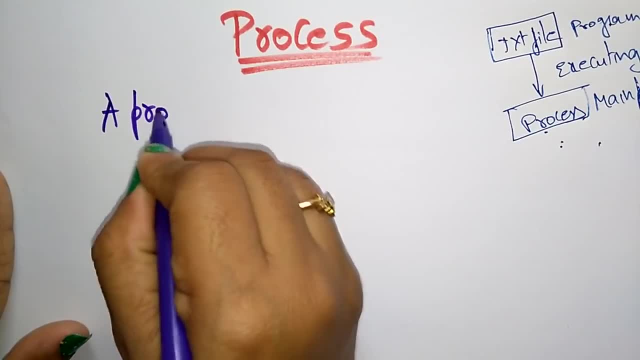 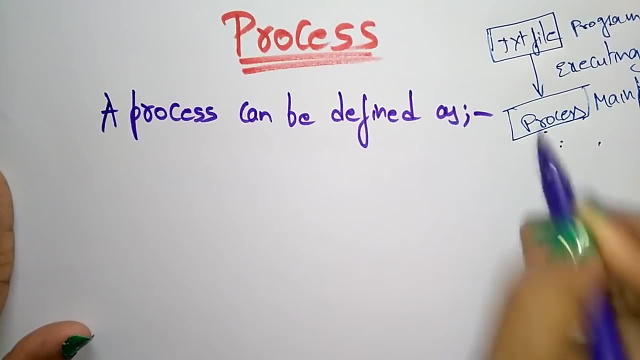 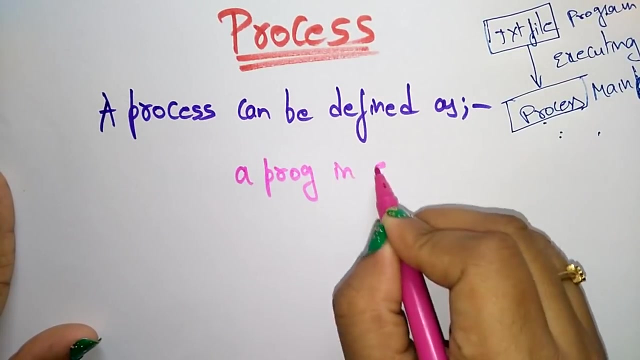 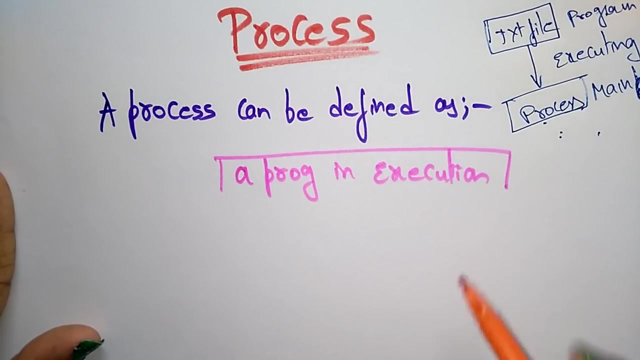 structure of operating system. So a process can be. A process can be defined as. So I am writing different definitions for the process. A process can be defined as a program in execution. You call that process as a program in execution or it is an instance of. 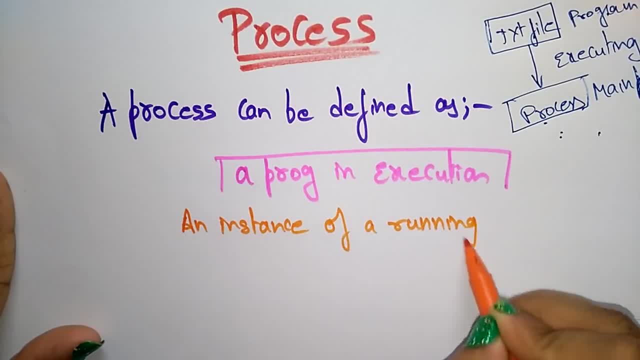 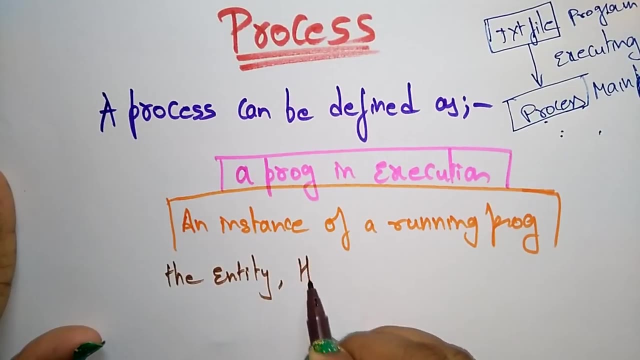 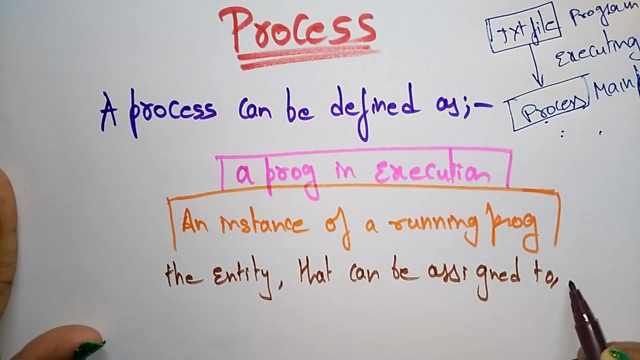 an instance of a running program. You call process as an instance of running program, or else a process is the entity that can be assigned, that can be assigned to and execute on a processor. okay, So these are the different definitions of the processor. 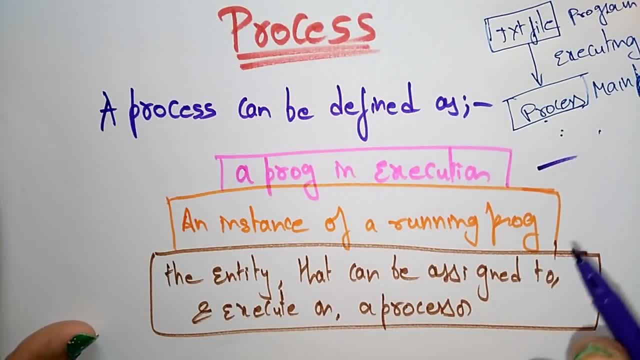 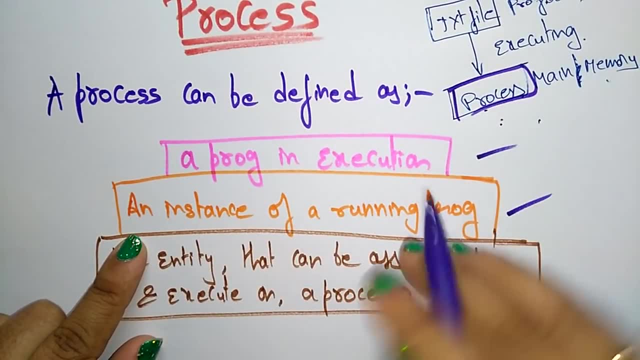 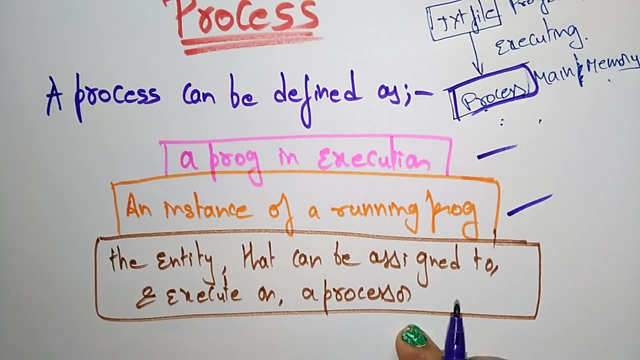 So a processor is a program in execution. You call a program in execution as a process. So an instance of running program so a running program. you call it as a process. or you just call an entity, So that entity which is assigned to a processor to execute the operation. 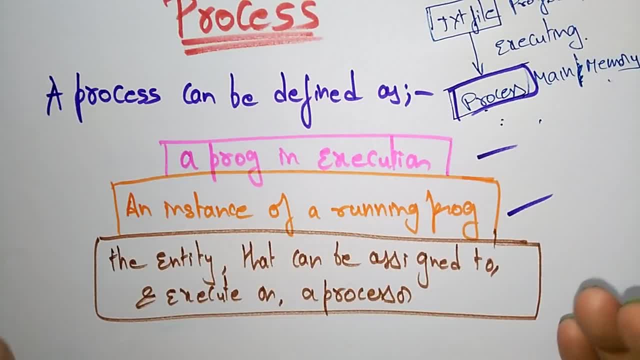 that parameter is assigned to a processor. So that parameter is assigned to a processor. you call it as a process means it is doing some work, it is doing some operation. it is it is giving some information to the processor. that you call it as a process. okay, so we can write a program. 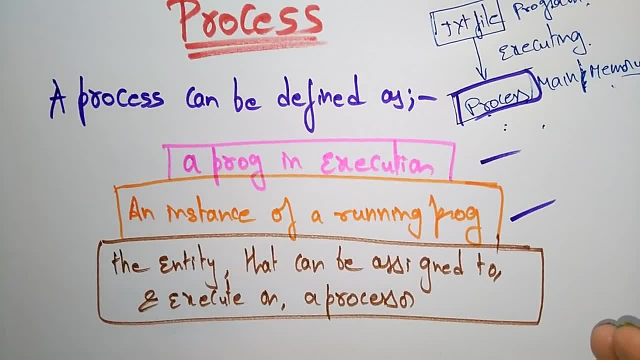 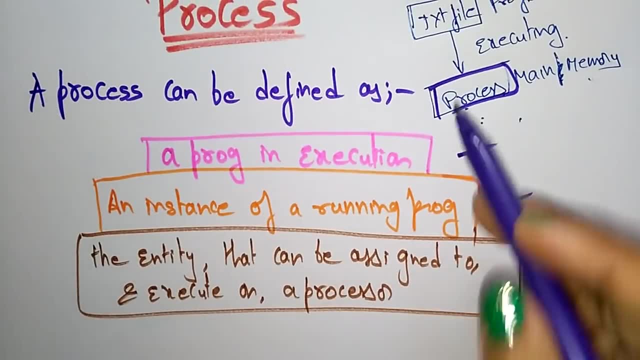 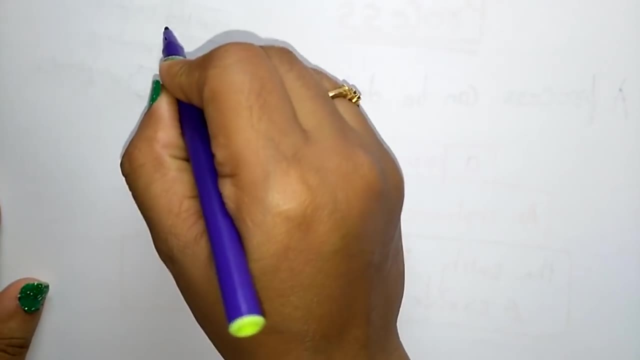 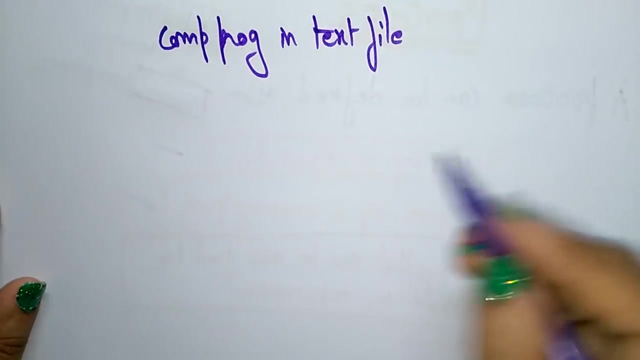 starting whenever we have taken that we, if we are writing a program, the program first it stores in the text file. so i already explained here, so here so a program. we, if you write a computer program, a computer program first we write in text file. okay, so when we execute this program, if you execute this program, 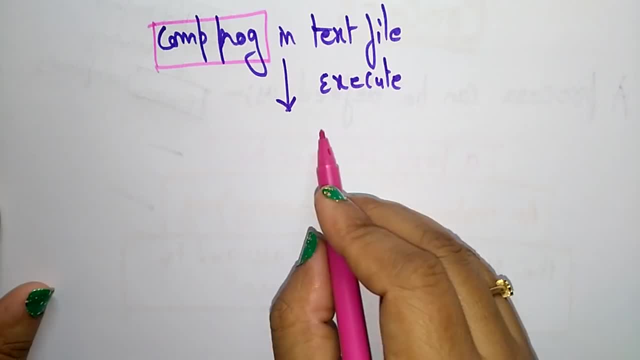 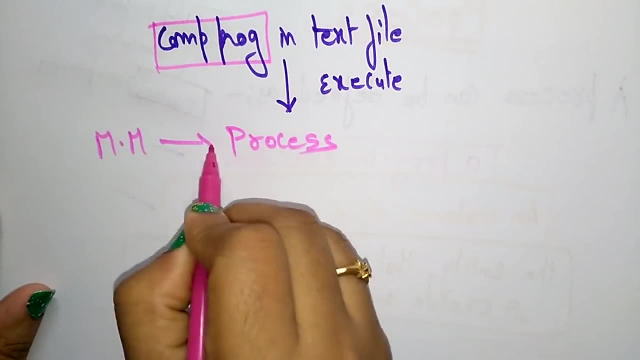 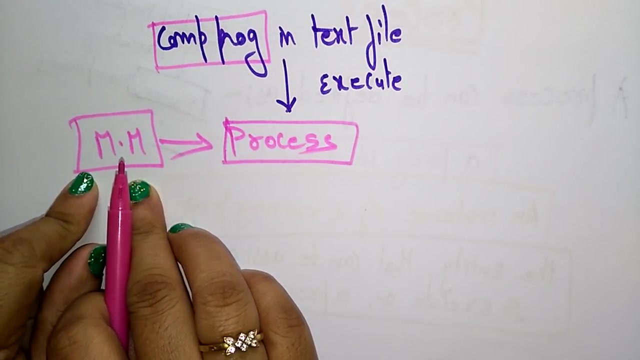 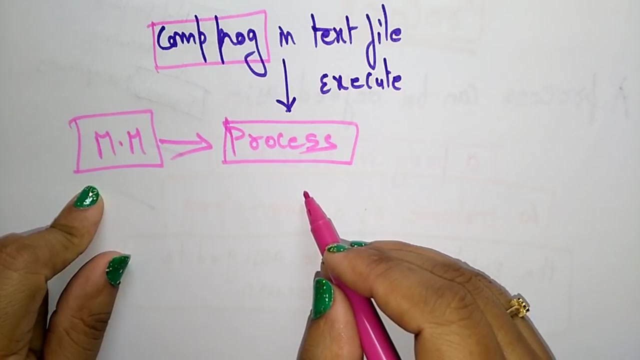 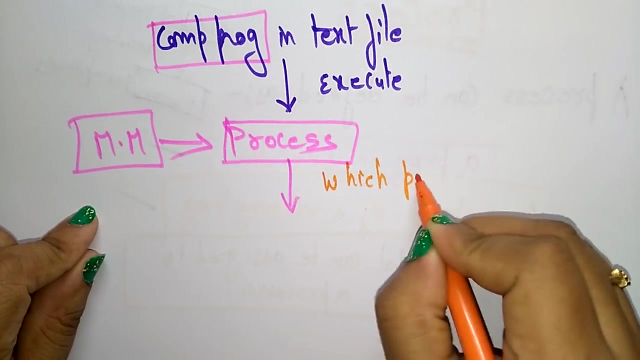 if you execute this computer program, it becomes process which is in main memory, which is in the computer program is become a process which is present in main memory. when a program is loaded in memory, it becomes the process, so a process which performs all tasks, a process which perform. 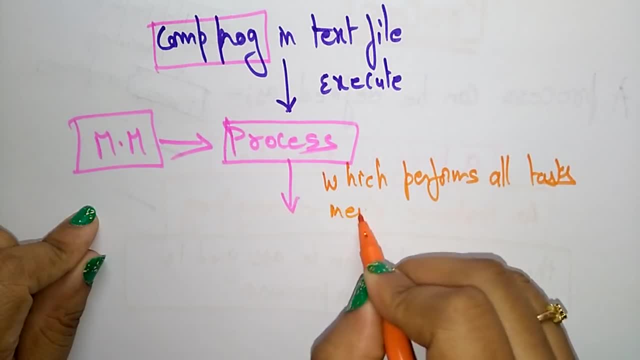 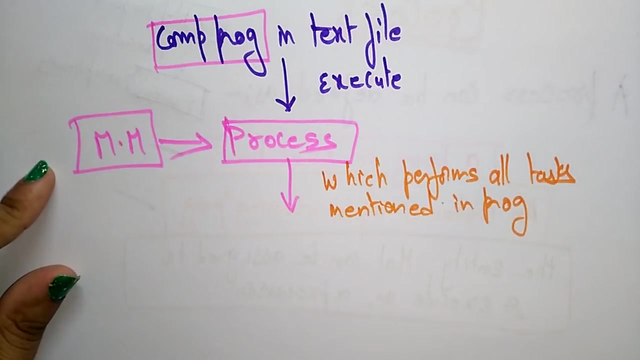 all tasks, many mentioned in the program. so, whatever the program, uh, consisting of the tasks that are present in the computer program, so that you call it as a process, a process which performs all tasks mentioned in the program. so those tasks will be divided into three types, sorry, four stack. 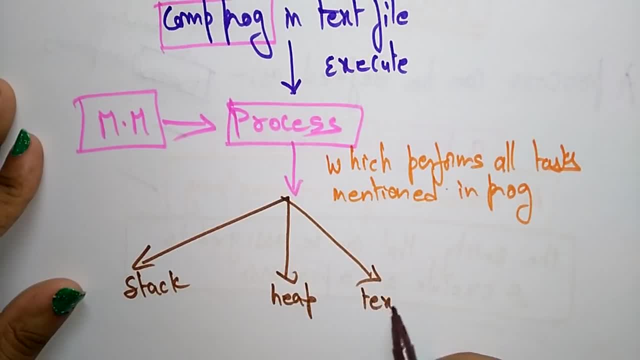 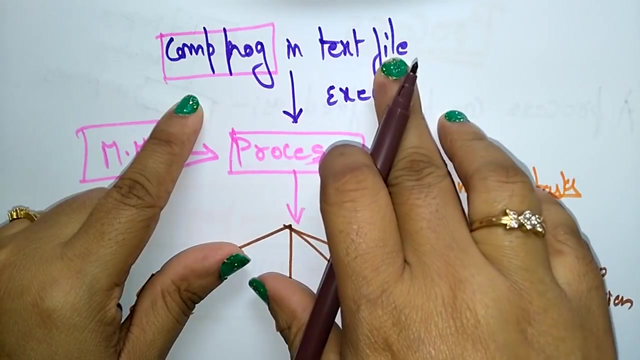 heap text and data. so the process is divided into, divided into four sections, so there is a stack heap text and data. so this is a simple uh, a process, a computer program, whatever we taken, that is written in text file. if it is going to be executed, uh, and it is stored in the main memory, then it becomes. 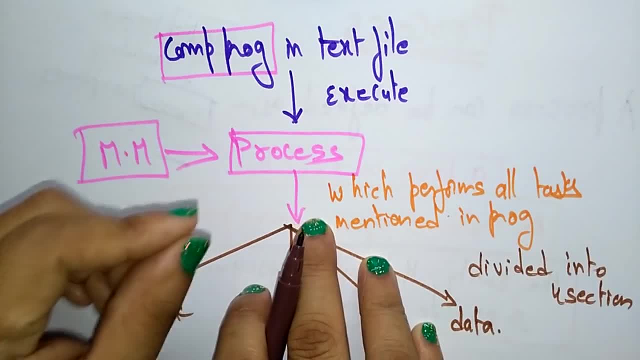 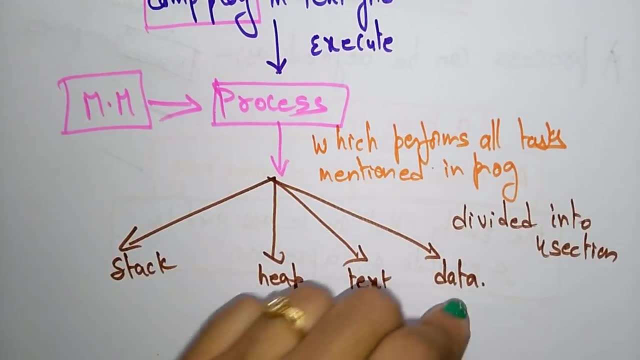 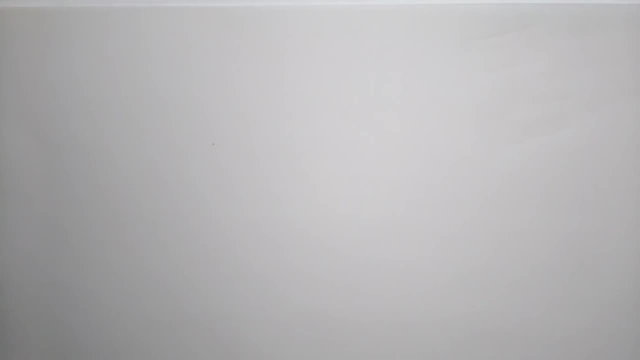 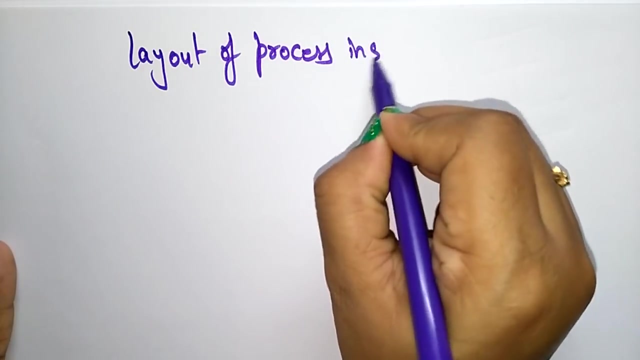 a process, a process which is performed, all tasks which are mentioned in the program. so those tasks will be divided into three, four uh sections, stack, heap, text data. so let me write the layout of this layout structure of process inside the memory, layout of process inside main memory. so let us take this is: